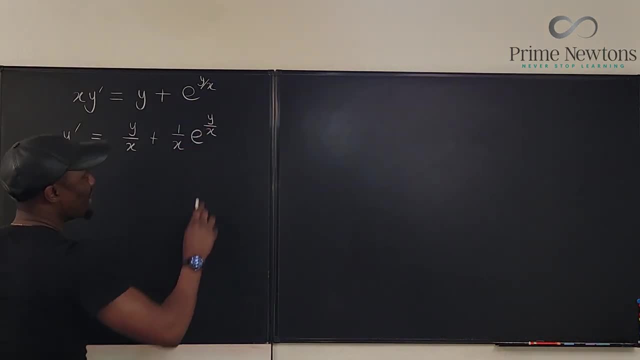 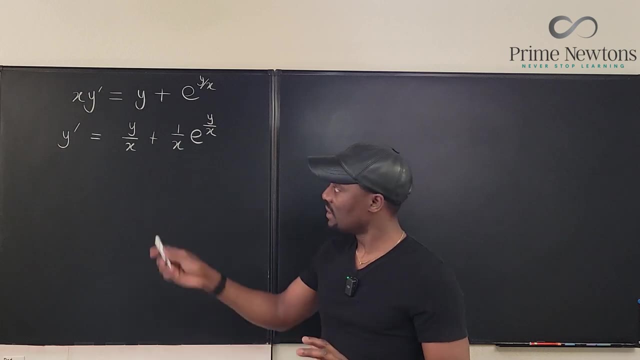 times y over x. So I'm going to write it as 1 over x times y over x. So I'm going to write it as 1 over x times y over x. Now, this question was designed in this manner so you could see something common. There's y over x here. There is y over x here. What can we do? Because there is no way you can separate y from x. So what we would rather do is, whenever you get this y over x situation, I would rather that you replace the y over x situation with the y over x situation. So let's worry a little bit about that. example: use x because it's got two elements, so I like being backs on this. Bring another variable So we meet and change it. I can't into x, I'm going to close the two form. so x is equal to y. 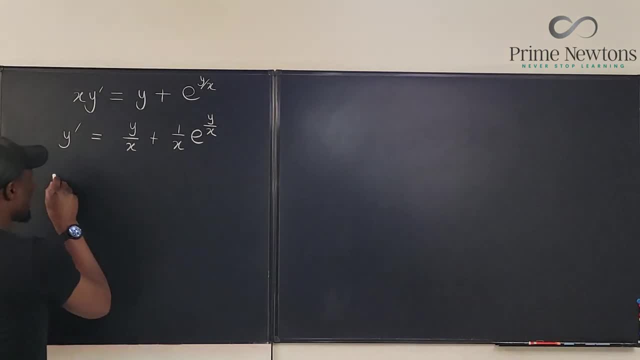 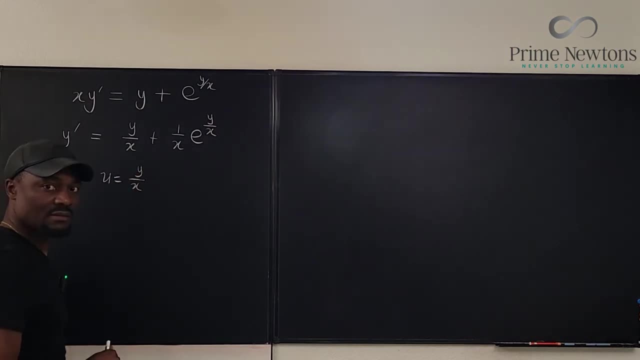 so we do a u substitution. So we're going to say: let's you be equal to y over x, and this means that y will be X, x prime. but you see, U is a function of x. So when you take the derivative of x fingers, the action is being replaced. 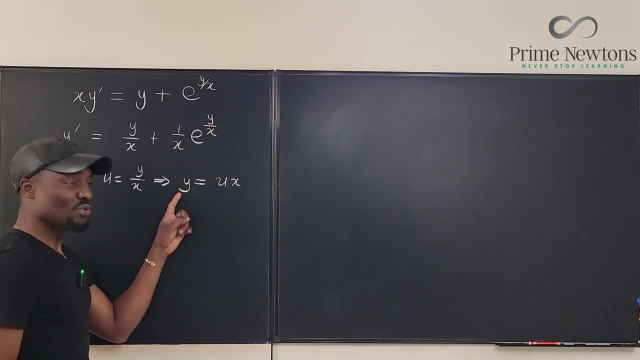 this you'll be applying, But this property over here. if I want an u, then u means a function over x. So when you take the derivative of this or the example cube, here u is going to be equal to x or the seulement bluff. 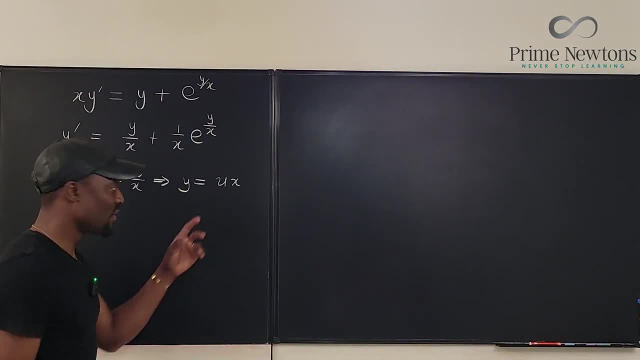 you'll be applying the product rule from Calculus 1 here. So we see that Y prime is going to be: we keep the first, we differentiate the second. If you differentiate the second, what do you get? You get one plus you differentiate the first U prime. 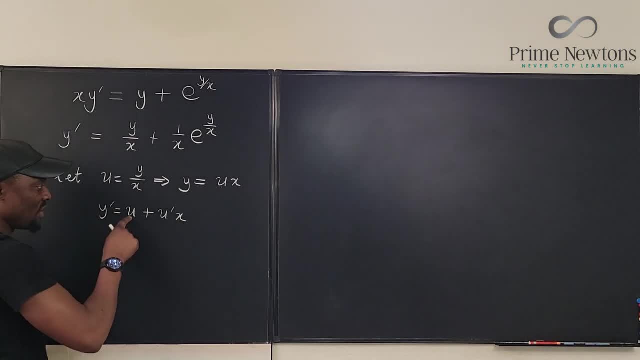 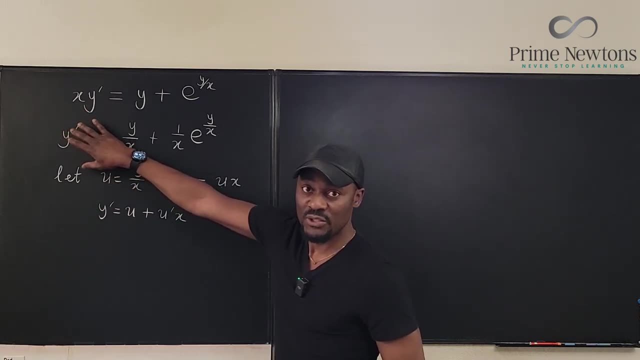 you keep the second X, So Y prime becomes U plus U prime times X. Now we're gonna go back to this equation and replace, do all the replacements that we can do. So let's go here. So we're gonna replace Y prime with this part. 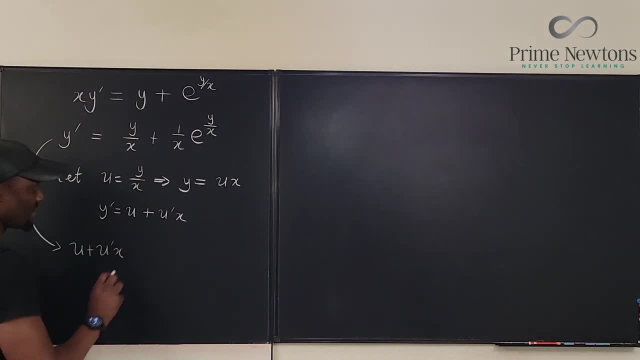 We have U plus U prime of X And we're gonna replace this guy with where is it With U? So that's gonna be one over X, And then this is going to be: there is no replacement for one over X. 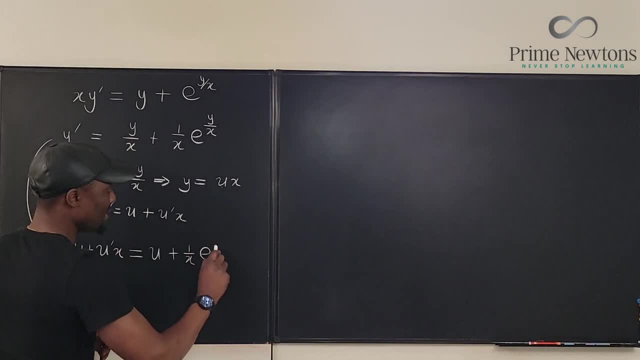 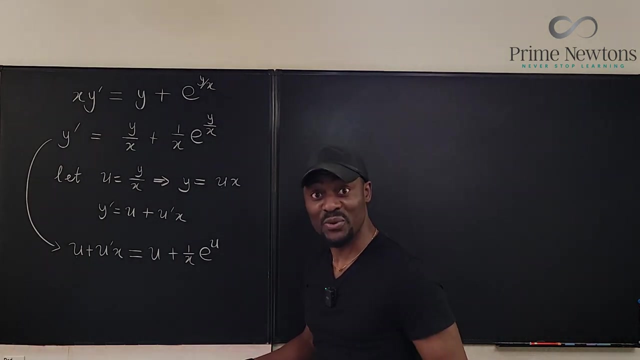 So one over X is here, and then we're gonna have E to the Y over X again is U. So this is what we have. But because this is an equation- you have U here, you have U here- You can cancel out both U's like that. 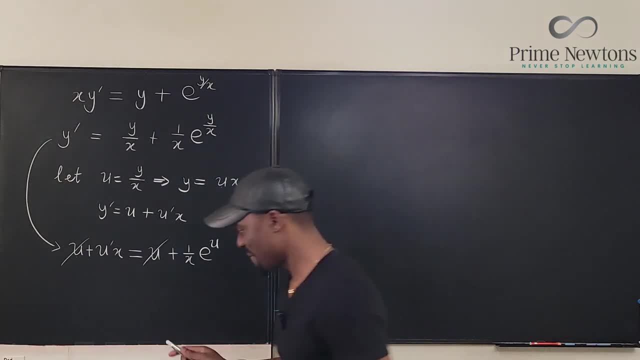 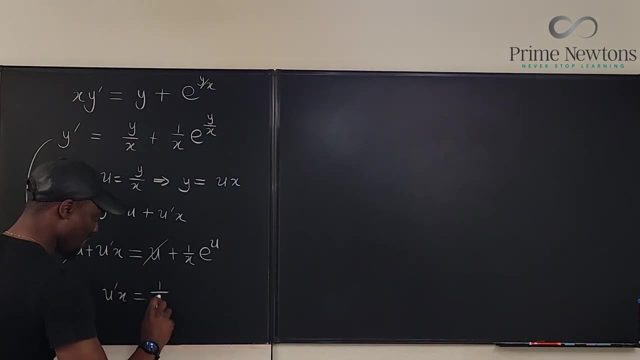 Cha cha. what do you have? We have U. prime of X is equal to one over X, E to the U. We can isolate this, So by dividing both sides by X, So that what we have next is just: you prime will be equal to one over X squared. 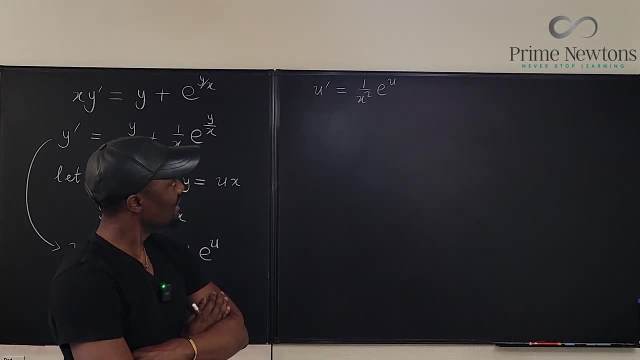 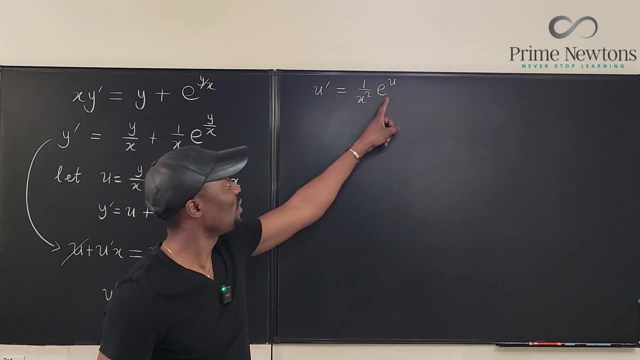 E to the U Nice. Now, once you have this, this clearly looks like a separable differential equation, because you can move this to the side. But before you do that, You want to rewrite whatever this is as du dx, It's better. 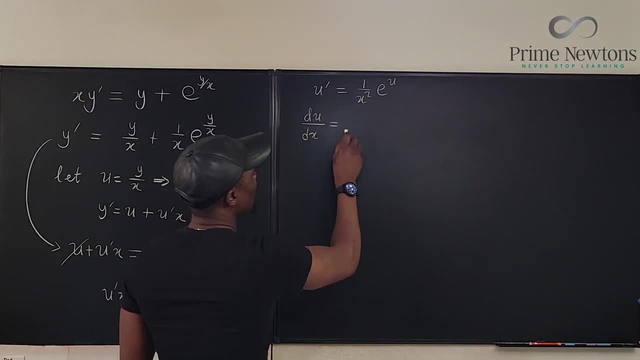 So we have du. dx will be equal to 1 over x squared e to the u. So now we can take the terms containing u, bring them here and leave 1 over x squared here. If I divide both sides this way, I'm going to have du, I'm going to have e to the u. 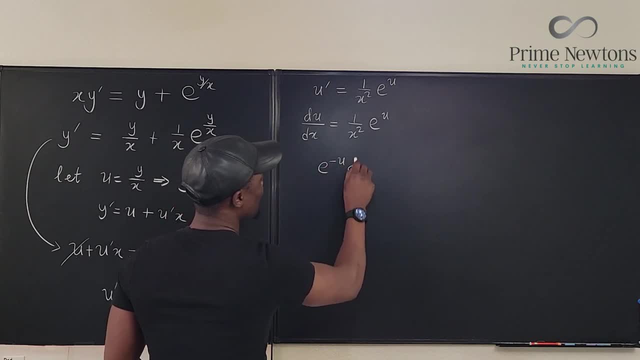 to the negative: u, rather du will be equal to what would this be? x to the negative: 2, dx. I've written both of them in exponential form. okay, in exponent form, So I can now integrate both of them. See, I multiplied by dx and brought this here. 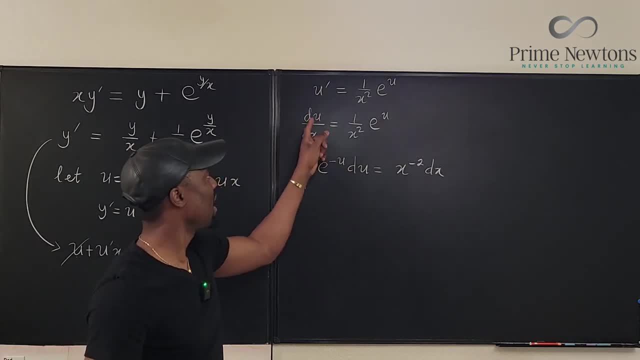 It became 1 over e to the u, which is u to the negative 1.. The du was still here, dx is here And I wrote this. It's this way. So now we integrate both sides. What do we have? 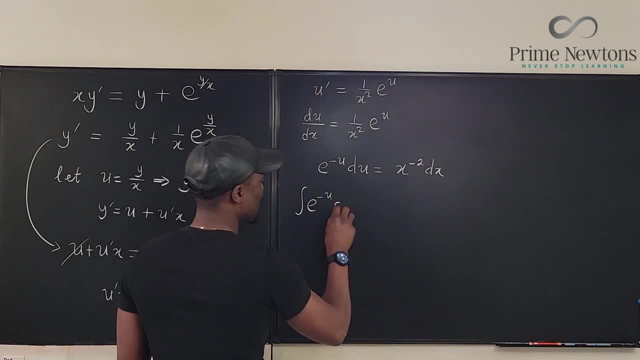 Let me write it here. So the integral of e to the negative u, du, will be equal to the integral of x to the negative 2, dx. So remember, if we integrate e to the negative u, it's just the derivative of this that's going to show up. 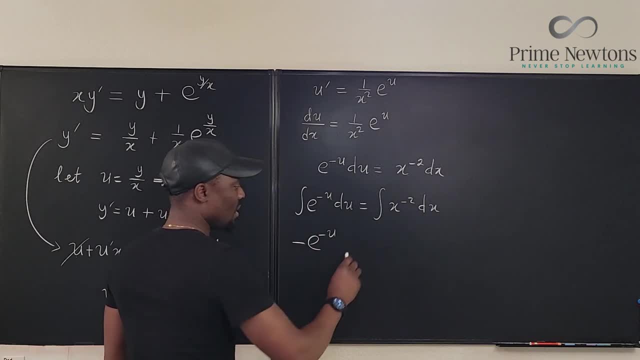 which is negative, e to the negative u. Okay, now should we do plus c here? Traditionally, we'll just add all the c's to the right, So wait until we're done. So here, what do we have? We have, if we integrate this, it's going to be x to the. add 1 to this. it's minus 1, divide by minus 1..